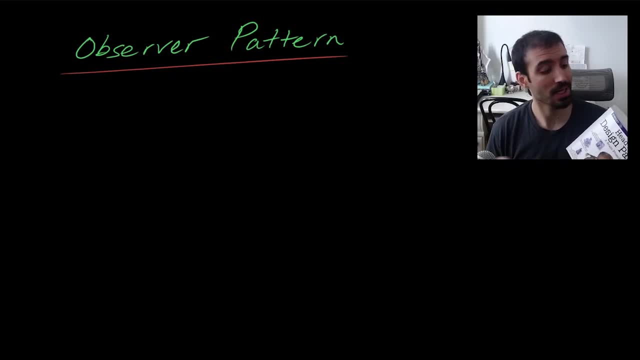 to be talking about the observer pattern, using this book as context. We're going to talk about what the observer pattern is. We're going to talk about an example of how it works and the different elements that are at play, And then I'm going to show you a class diagram to demonstrate how it. 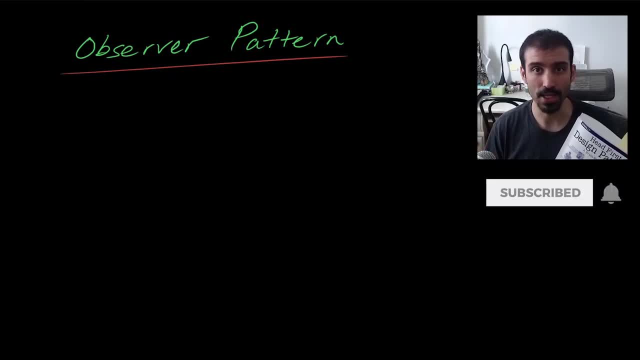 could potentially all fit together. And then, finally, we're going to go into my IDE and I'll show you a real example of the observer pattern in real life. So that's the agenda for this video. So the first thing that we are going to do is define the observer pattern from this book. So 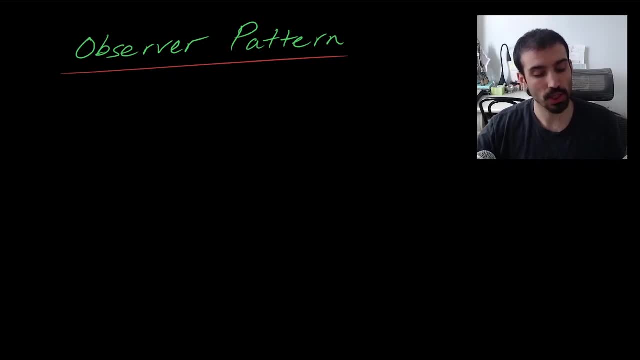 the definition of the observer pattern is as follows: The observer pattern defines a one-to-many dependency. So one-to-many dependency, So one thing and multiple things that are dependent on it, between objects, so that when one object changes state, all of its dependents are notified and updated automatically. So I'm 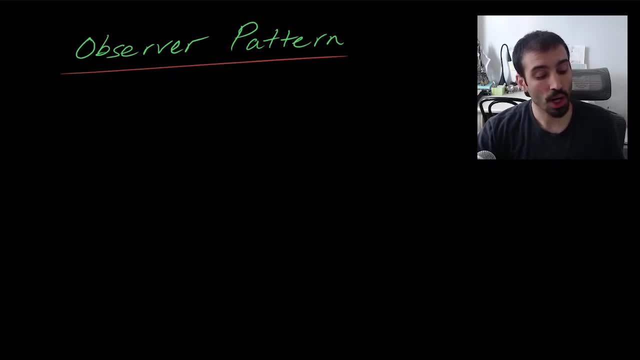 just going to repeat that last part to you because it's kind of important: When one object changes state, all of its dependents are notified and updated automatically. So let's break that down a little bit. So we have one object, one object that is kind of the, the subject or the core object here. 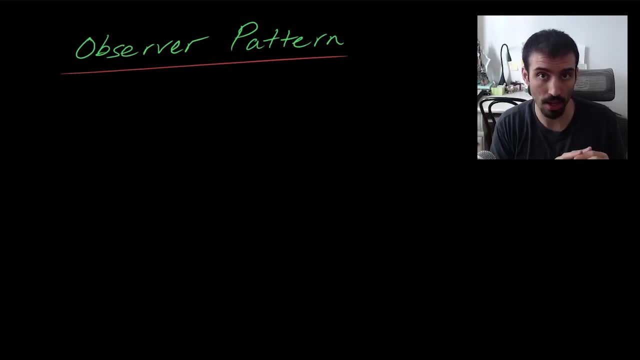 And we have multiple different dependencies that care about that one object. They want to know when something happens And the way the observer pattern works is that on that one object, whenever something changes in it, the change is propagated to all the dependents that are interested in that object. So that was a whole bunch of words, So let me draw out an example. 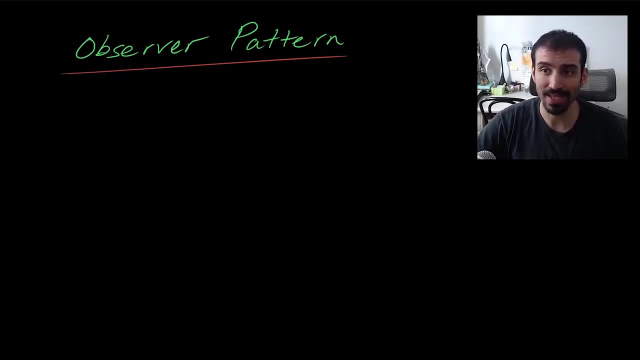 Here that we're going to be using throughout this exercise, just to demonstrate exactly what I mean by this. Okay, so assume that we have a weather station, A weather station, Weather station, And we'll just denote that by this circle here. Let me just round that out a little bit. And this: 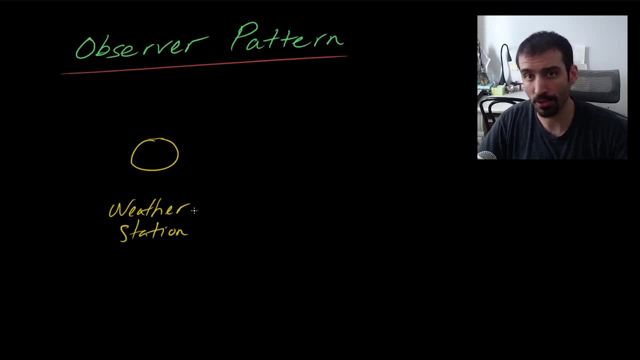 weather station. its job is just to collect some basic information. You know a typical weather station does. It collects things like humidity, temperature, wind speed, all that kind of stuff. So this thing is collecting all these three things. So in this example, this is the one in that one to many definition that we just spoke about. Now this 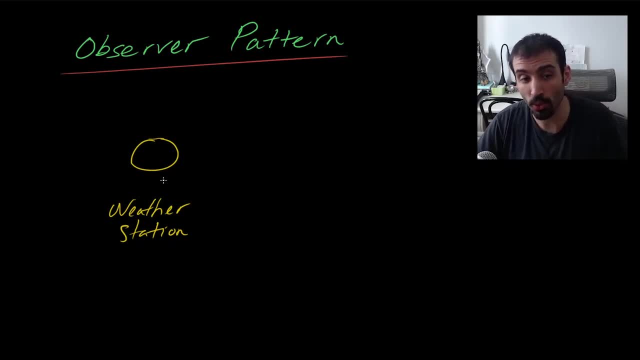 weather station, since it represents the one, The one in the one to many relationship. It's what's called the subject, And there's a lot of different terms. Sometimes people use the publisher or the topic, But I'm going to be using subject, because that's what they talk about in this book. So the 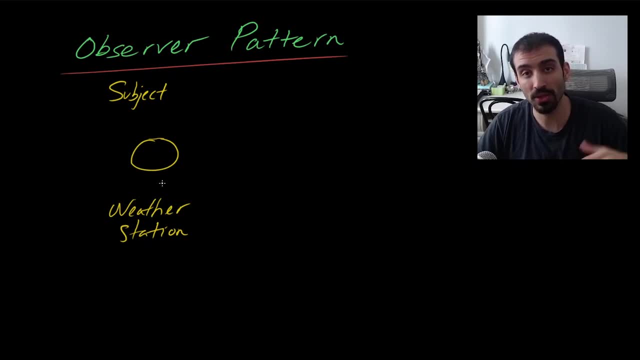 weather station is the subject. So whenever something changes about the subject, that needs all the other dependencies. So the weather station is the subject. So then, what are the observers? So that means we have to have many observers over here, Right? So let's just say: 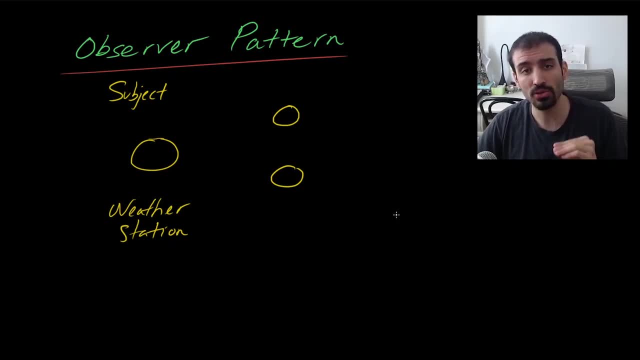 there's two different observers And let's say that these two observers are interested in getting the most up-to-date temperature and humidity information that this weather station retrieves. Say, this weather station does that once every hour, or something like that, And these two observers only care about when something happens. So say for this first observer, its job is just to. 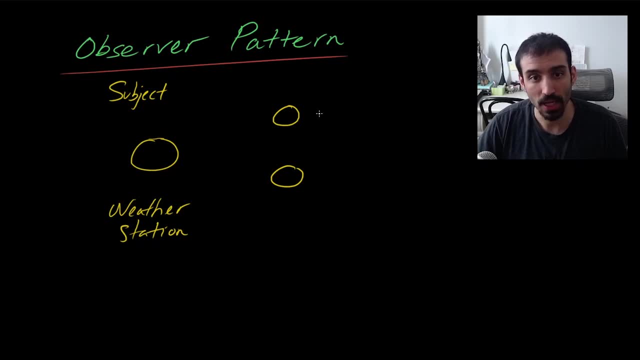 maintain whatever the current temperature and current humidity is. So let's just call it the current display, Because it's displaying the current information. So, again, like I said here, this is the subject And these are going to be the observers. Let me just fill. 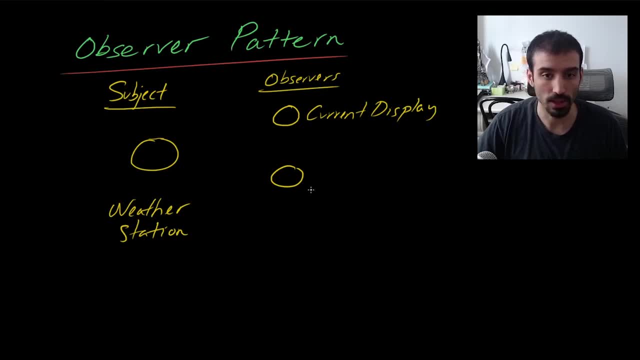 in everything here, so this all makes sense. Okay, that's looking good. And this second one here, The second thing that cares about changes in the subject. Maybe this is for forecasting, Because it wants to keep track of all the historical information of as this weather station changes. 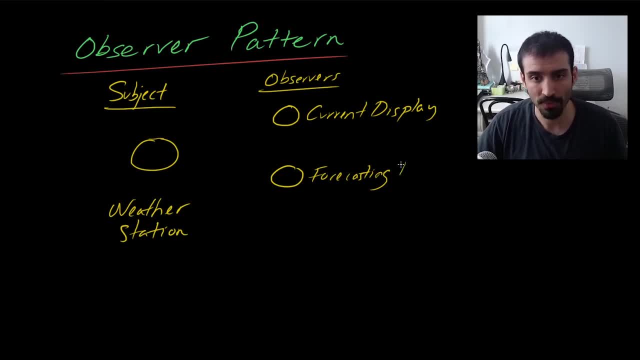 and then maybe output some kind of forecast or prediction or something like that. So this makes sense. so far, Right, It's pretty pretty reasonable. So in the observer pattern, just to recap, you have the subject, which is the holder of state, the holder of information or data, And then you have these: 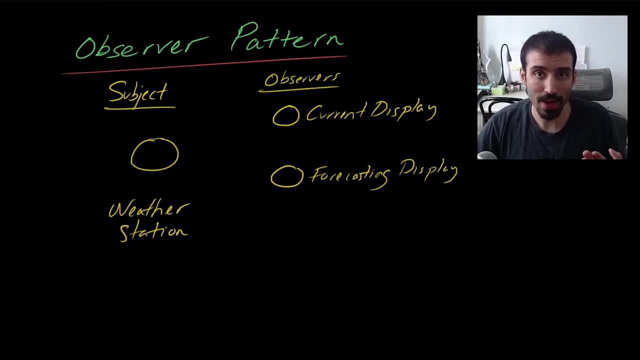 observers that care about that data. So in the observer pattern you have something that's called a subscription, So the observers need to form a subscription with the subject. And think of this like registering to go on a mailing list. Like if I want to be on a mailing list, I need to register my email to that mailing list so that I'll. 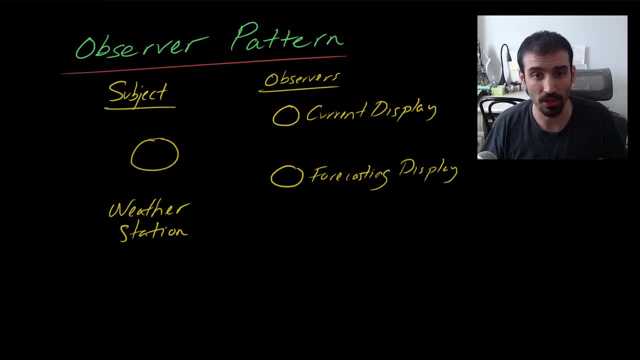 receive an update whenever the person sends an email. Exact same example here. So the observer registers with the subject, But the arrow actually goes in this direction, because this is the data flow direction: It goes from the subject to the observer, But the registration actually happens. 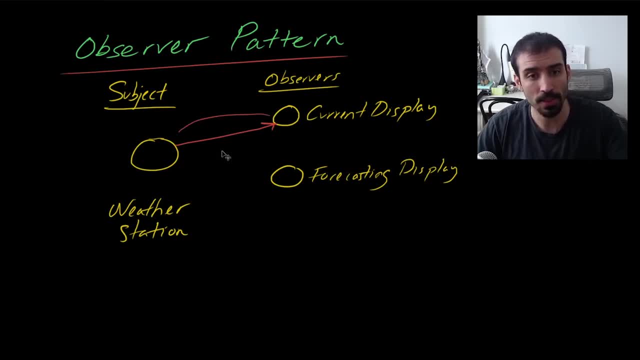 in the inverse direction, like that arrow that I just drew, But just to demonstrate data flow. I'm just going to keep it going in this direction. So these are subscriptions- Subscriptions- I'll just call them subs for short, And so the way the observer pattern works is that whenever 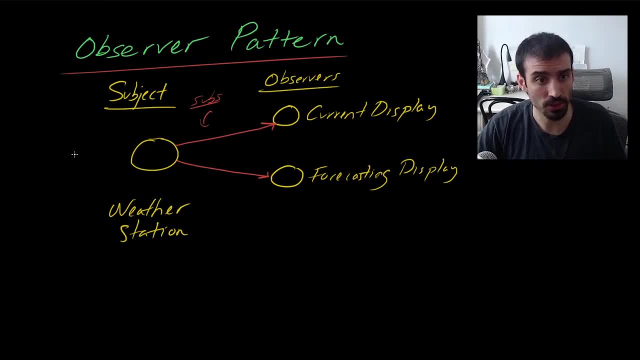 something changes on the subject, in this case the weather station. So say, like every hour ticks and it's doing an update, So new data gets populated into the weather station. The subject will broadcast a message to all of its observers. So one subject broadcasting a message to all of its. 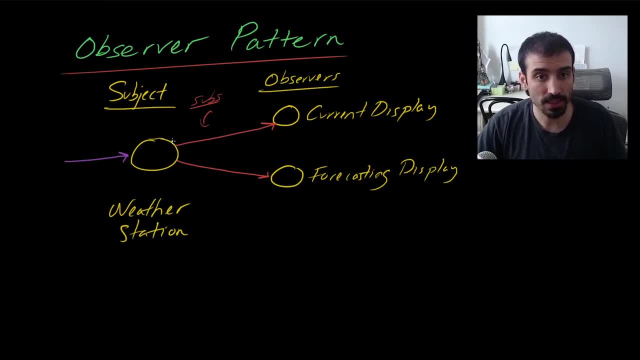 observers. So when something happens on the subject here, data gets sent to this observer in this line and this observer in this line. Now there's multiple different ways of handling this. In the software world it's usually you have like an update function in the current 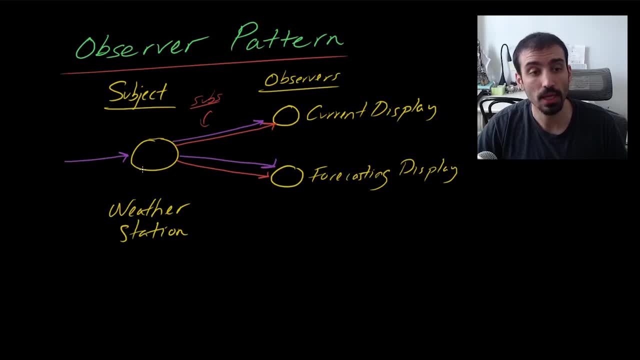 display and that update function gets called by the subject. That's generally how this works. And then in that update function you have like a handler that does whatever it needs to do whenever the data changes. In the case of the current display, all it probably does is sets a local. 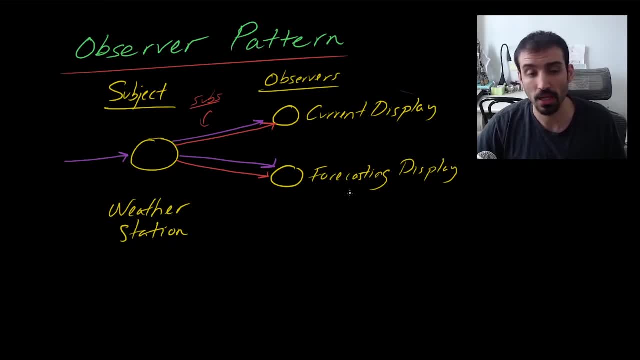 variable In the forecasting display. all it probably does is, you know, set a list of all the historical things and then maybe it needs to save that to a database or whatever it needs to do. So this is the idea of the observer pattern And this idea how you have one topic, one subject. 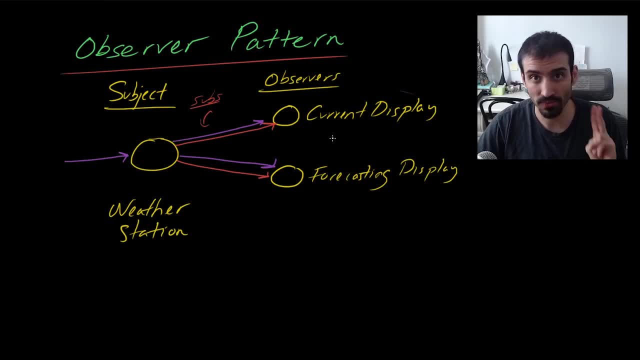 and multiple observers. it's also called fan out. fan out because you have one entry point and multiple different kind of tangential flows that it can flow into, to kind of update this data. So this is the observer pattern. So let's quickly talk about like why this is a good and useful 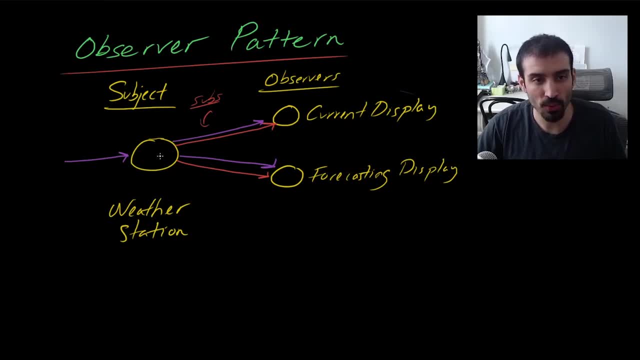 thing, And let me just get a different color to denote Here, So we know that when data changes it flows to all these different observers. So say we did this the other way around, say the observers were responsible for getting the data from the. 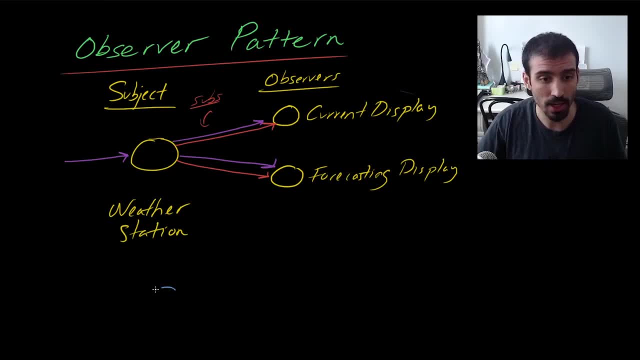 subject. So, instead of having what we have here, we had a thing where you know we have these three different circles And now these guys are polling, and polling just means like calling on a timer and frequently asking: Hey, did anything change? Did anything change? Did anything change? If you think. 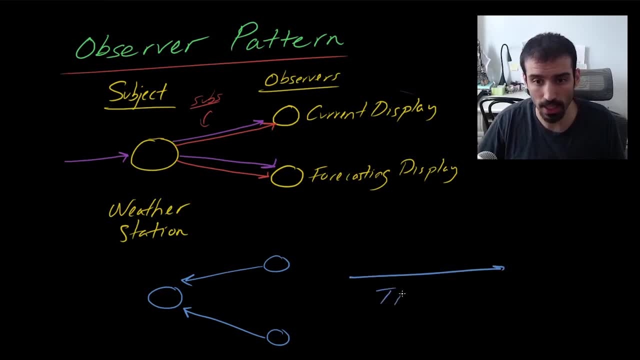 about this like over a timeline say. this is a timeline, That means that every observer- and we have two observers here and kind of this timeline corresponds to whenever updates happen on this subject, So maybe new weather updates. So let me get a different color. 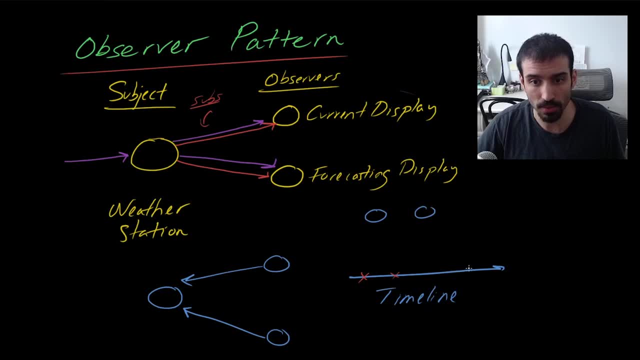 actually. So an update happens here, an update happens here and maybe an update happens here- I don't know something random like that. So if you weren't using the observer pattern, how would these guys get updated whenever something changes on this weather station? Well, they'd have to implement some kind of 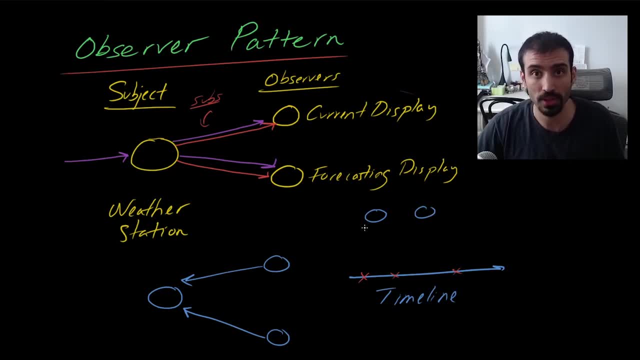 polar, something to do on a timer to constantly check the weather station over and over again every few minutes. so it'll be asking over here and maybe asking over here. then it maybe asks over here. oh, I found a new one. And then it finds a new one and does. 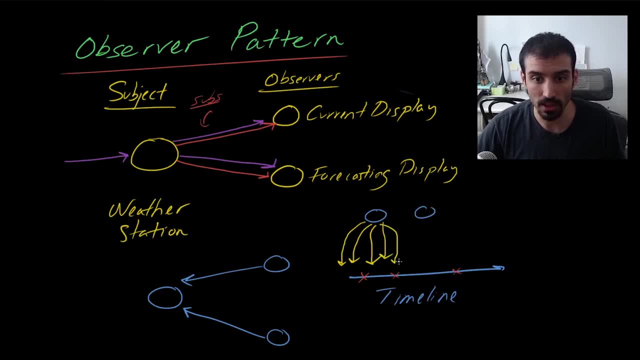 something with it And it keeps on going, asks over here, then ask here- oh, I found a new one- then it keeps on going. So you see, there's a lot of wasted cycles here in these observers, And these wasted cycles are multiplied by the. 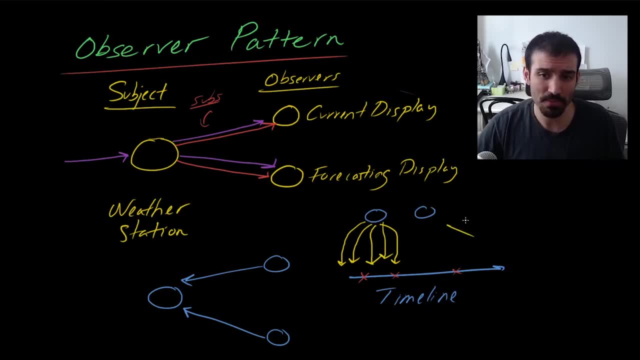 number of observers you have. So this is a very bad pattern for the observer being responsible for retrieving the data. And when we think about this from the observer pattern perspective, which is the opposite, which is this example over here, all we have is one update that's occurring. 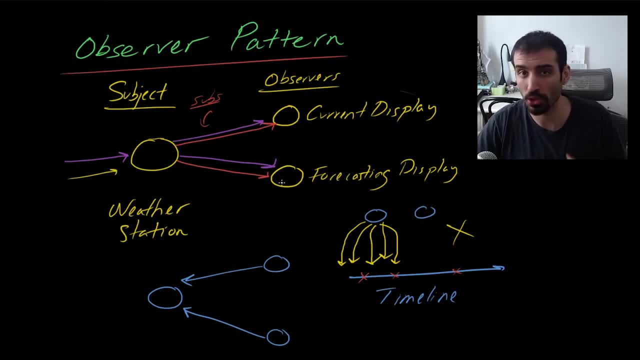 and that's getting automatically pushed into all the observers. So no polling, no wasted cycles, no, nothing like that. So that's the most practical reason of why the observer pattern is useful. It's also useful from just a general best practice perspective. 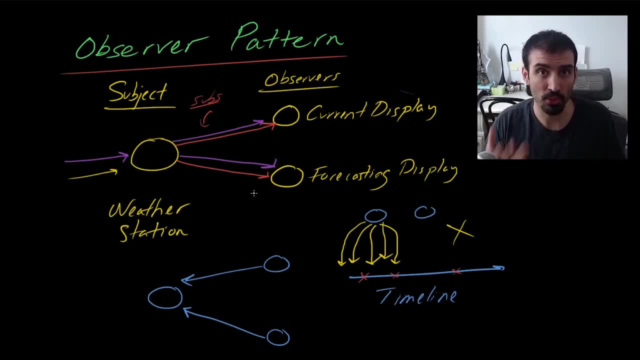 It's great for a loose coupling, So it allows systems to kind of operate independently. And what I mean by that is the subject here doesn't necessarily need to know about the observers, So the subject can operate independently and the observers are the ones with the dependency. 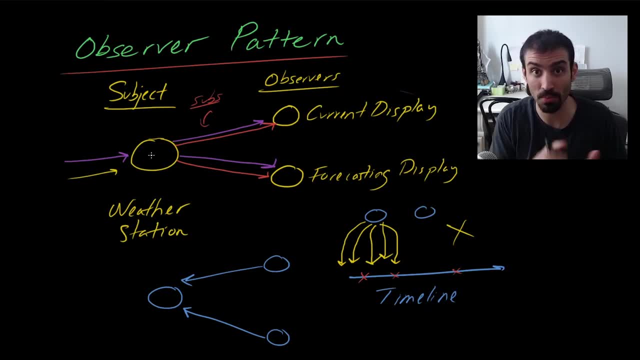 So that's one of the benefits. That means that the subject and observers can change independently in terms of software upgrades, in terms of anything that they wanna do in their system. Another good reason, another reason the observer pattern is useful is because it's great for testability. 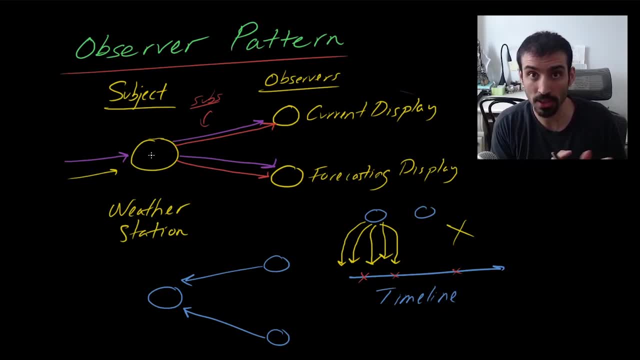 makes systems easier to test when you're only testing a single component, and the less dependencies that you have in a system, the easier it is to test it. So that's another main benefit as well. You see this pattern all over the place in a lot of different libraries. 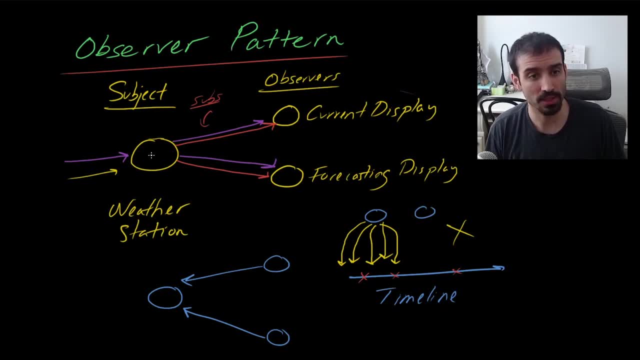 especially for like thread pool monitoring and stuff like that, at least in the Java language And in the system design perspective. you see it a lot in cloud systems, So AWS SNS is a very popular implementation from a system design perspective or an architectural pattern. 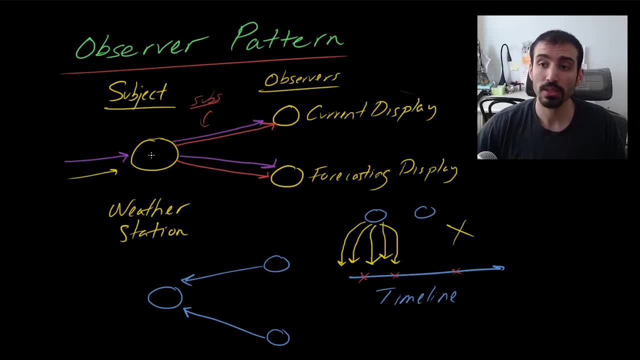 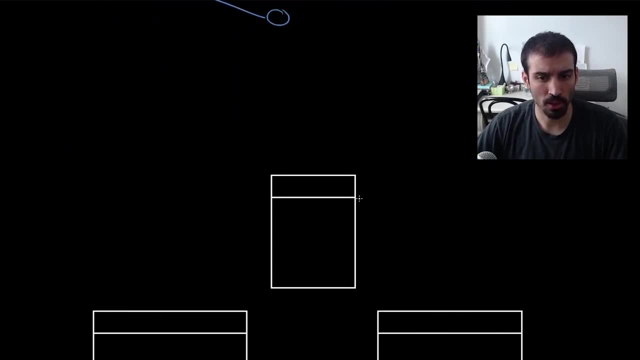 What we're gonna be talking about in this video is more in terms of software. So that's what the observer pattern is. I hope that was clear to all of you. Let's go down to my class diagram section where I'm just gonna kind of break this down. 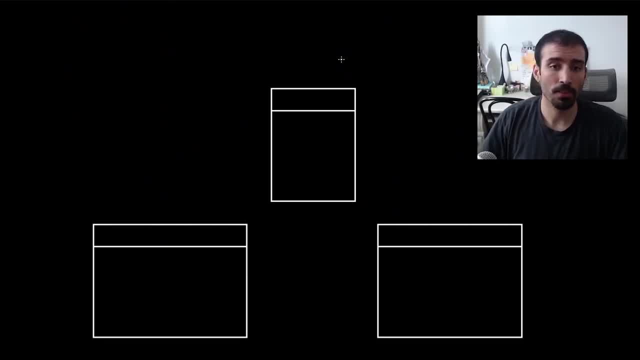 in a practical example, just using some classes here. Okay, so the first thing that we need is we need to kind of represent the subject or the topic. In this case, it's gonna be the weather station example that we were just discussing. 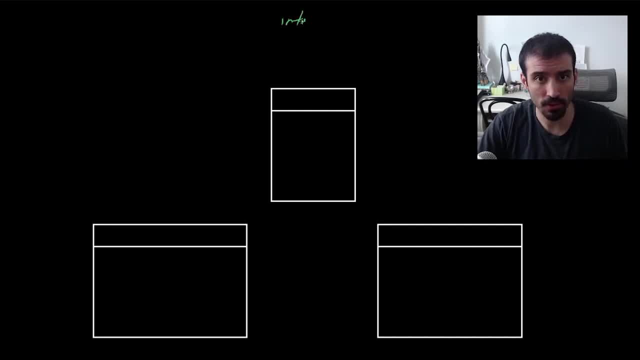 So let's define a interface. So we're gonna have an interface up here, interface, and just put some brackets around it And we're gonna call this interface the subject. Okay, and subject is gonna be the thing that broadcasts the messages out. 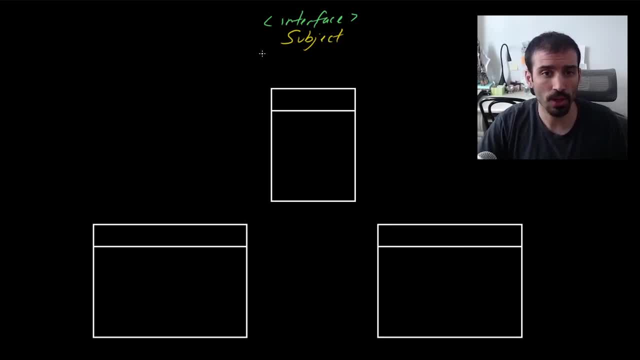 And this interface is gonna have a couple methods. The first one is gonna be called register- register observer- you can possibly call it. Another one is gonna be called the remove- remove. And the last one is gonna be called notify- notify. 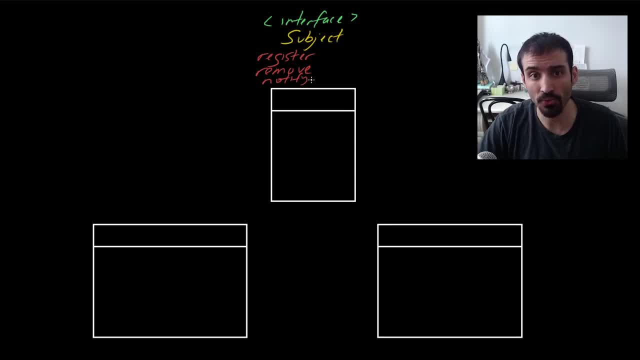 So: register: adds an observer, remove, removes an observer and notify: broadcasts a message to all the different observers. So those are the methods that this thing uses, And then we're gonna have a concrete class called weather station, Weather station And the weather station- we're gonna put this in purple. 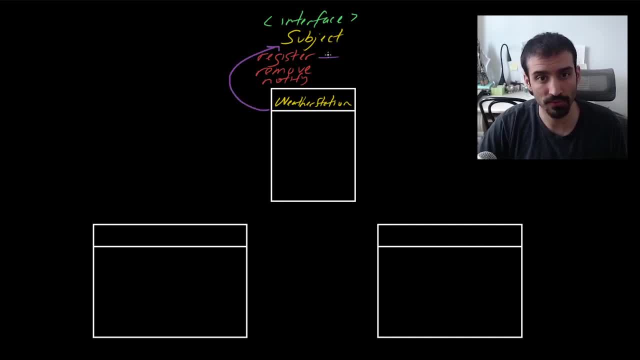 is going to implement the subject interface, So it's gonna have to define all these three methods that exist here in the class body. So that's good for subject. We're also gonna need a separate interface to represent the observers, So we're gonna create a observer interface. 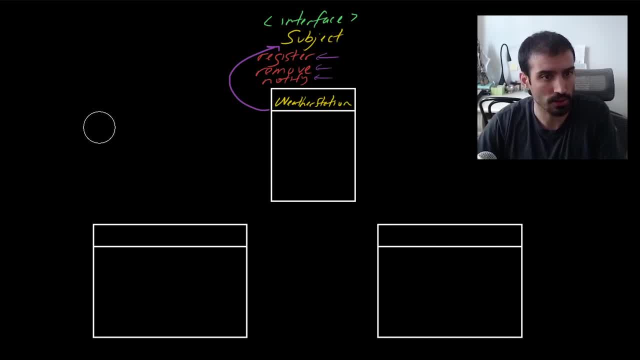 So we're gonna call this observer. Oops, actually this should be. oh yeah, so it's just interface here, Interface, and we're only up to interfaces, So don't worry if you're getting tired of this. So the interface is gonna be called observer. 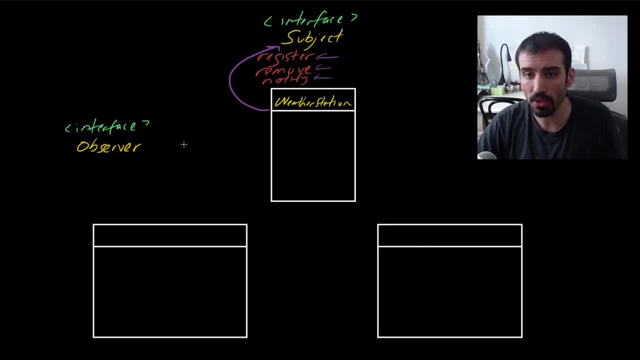 And I apologize in advance for my horrible writing- And for the interface. all it's gonna have is one method, which is called update, update, And for the observers, they're gonna implement this update method because that's what's gonna take the data. 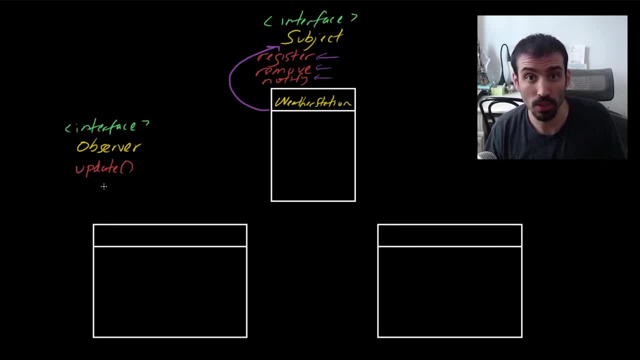 And for the observers, they're gonna implement this update method because that's what's gonna take the data, So it's gonna tell the weather station what it should do with this observer when a change event happens, And we're gonna see that more in a few moments here. 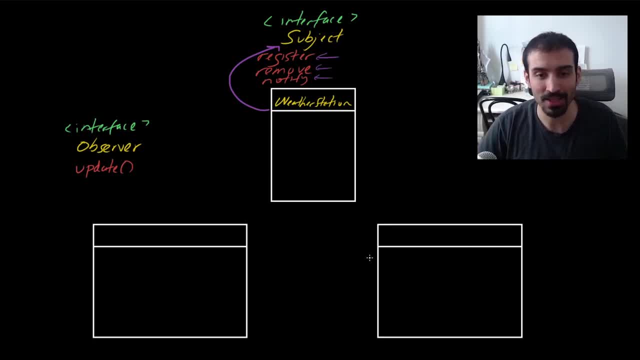 So let's just fill out the remaining class here and then we can get the remaining classes rather then we can get into the actual implementation. So in this example I think we said we have a current conditions display, or current, let's just call it current conditions. 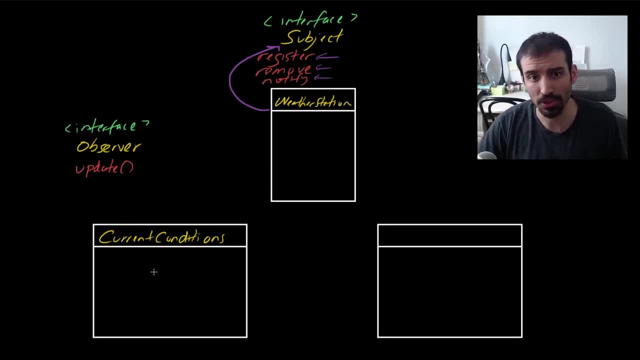 And this thing's job is just to keep track of the current temperature and current humidity. So we're going to put temp and humidity And maybe it wants to store it over time or something like that, but that's basically all this thing is going to do. 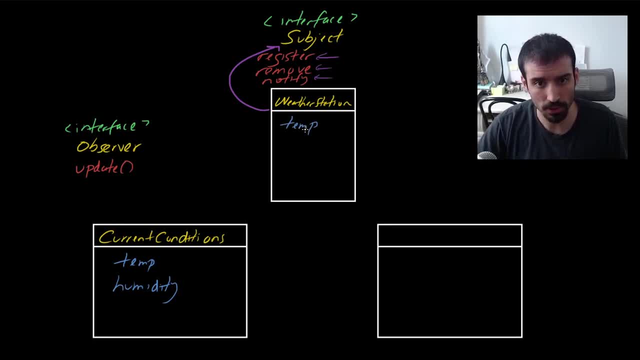 Oh, by the way, the weather station also has these properties. It has the temperature and the humidity, But again, this can change over time as the weather station continually makes measurements. So that's what we're going to have for the current conditions. 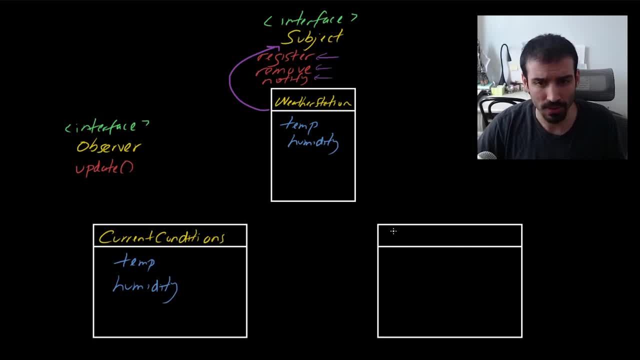 And then we also have a second one. I think I called it forecast. It has forecast conditions. I apologize for my horrible writing And this thing is going to. I'm not going to write it here, but it's just going to maintain the history. 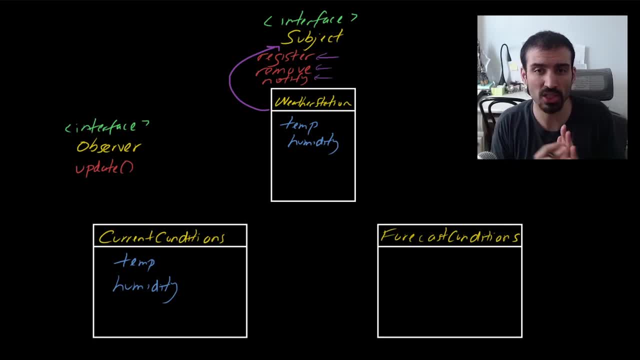 of all of these different temperature updates and then just expose them in a method. Maybe you'll have a method that says like: display last seven days or something like that. So let's put that here, Last seven days method, something like that, And then maybe 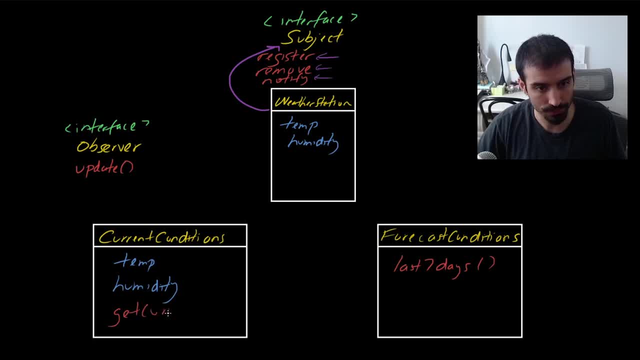 Maybe the current conditions. one has something called get current. So that's the idea here. And then with this interface, these current conditions classes are going to implement this interface. So that's what we got going on here. So just to kind of recap what we did here. 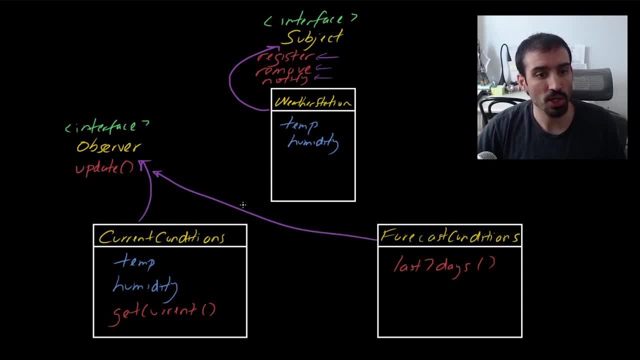 So we have a weather station that is going to be our subject. We're going to register these current conditions, concrete classes which are of interface, observer, And whenever something changes on the weather station, whenever there's an update to the temperature or humidity. 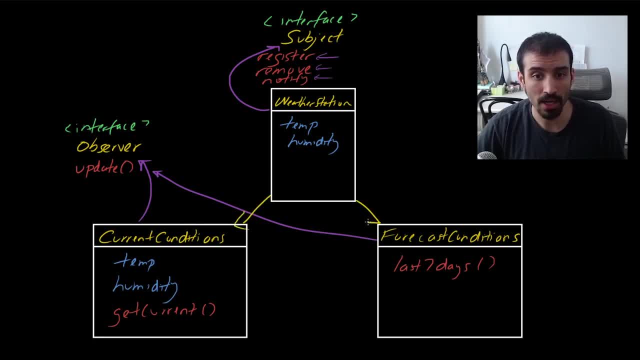 we're going to propagate that update into this class by calling the update method And that's how that fan out happens. So whenever something changes on the weather station, that's going to call all the observers update method And that's where the observers are going to kind of set local variables. 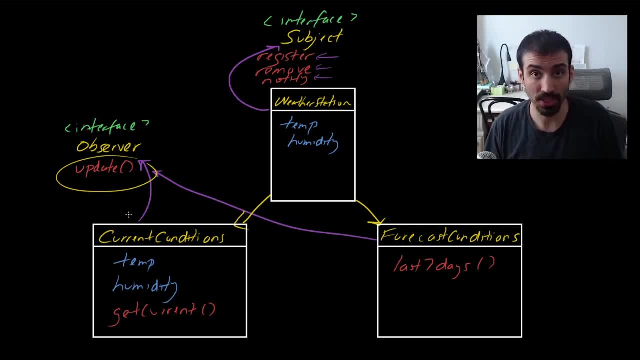 or do whatever they need to do. So that's what we're going to be doing in the implementation. Now I'm going to switch over to my IDE, So just kind of keep a frame of reference here, because this is what we're going to be implementing, or what I actually already have implemented. 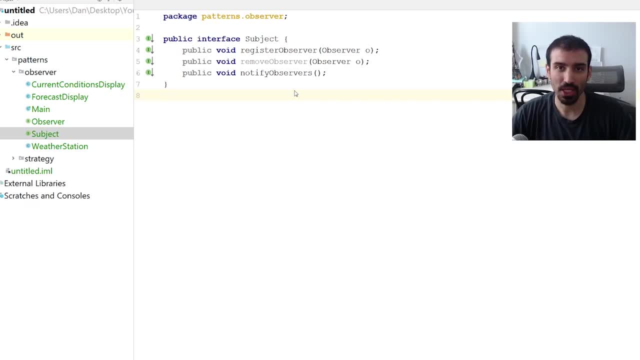 So I'm going to show you how to do that now. So let's switch over, All right guys. So here we are in my IDE. So first of all, let's just take a look over on the left here of the project structure. 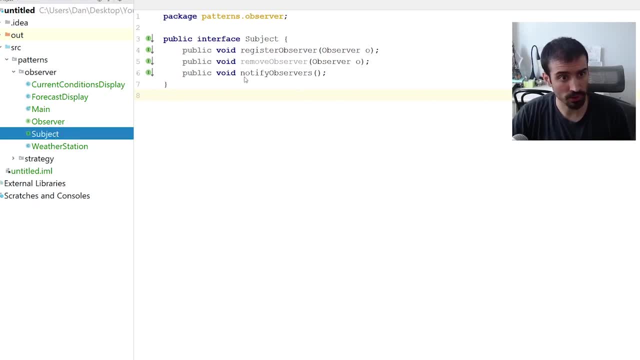 So we have the subject interface, which is what I described and actually what I'm showing on screen Now. we have the observer interface, which contains the update method. We have the weather station object, which holds the temperature and the humidity, at least what it is whenever it gets measured. 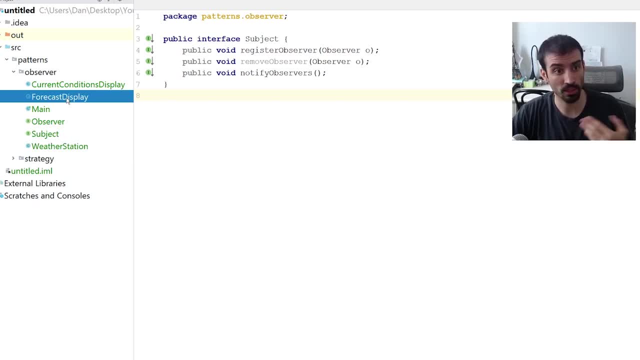 We have the forecast display, which has that seven day average thing where it can get the seven day average of temperature measurements, And then we have the current conditions display, which just displays whatever the current conditions are. So that's the idea here. 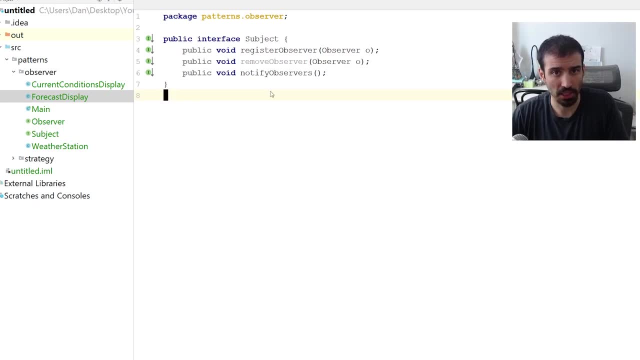 So let's go through these classes one by one. So we have the subject here And, like I said, we only have three methods that we really need. So first of all, we're going to have a registerObserver method and that's going to take in an observer. 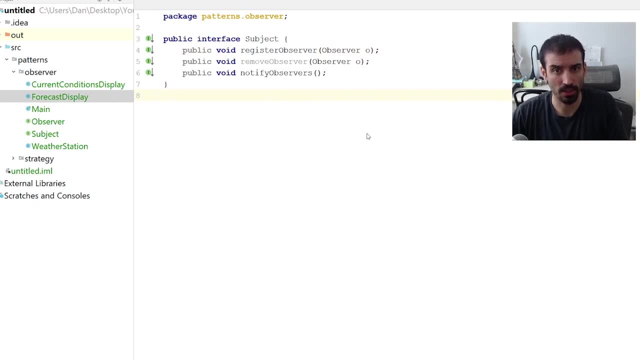 obviously. And then we can have a removeObserver method, which is going to take in the observer as well, And then we're going to have another method called notifyObserver, that calls the update method for all of the observers. And then, third, we're gonna have 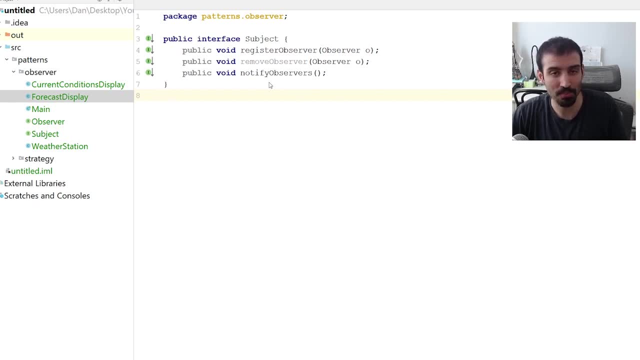 this notify observers method, which basically triggers the updates in all of the different observers so they can effectively get notified whenever something changes. So now let's look at the observer, which is very, very simple. All it has is one method, which is update. 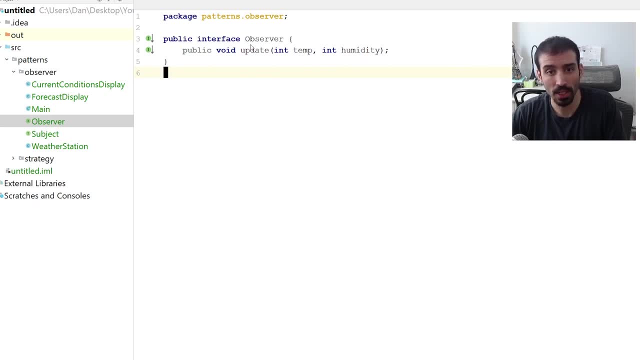 and that takes in the temperature and the humidity. So the update is gonna occur. You're gonna take these two things in and do whatever you want with that data Whenever the update is triggered. that's the new measurement of the weather station, So let's keep on going. 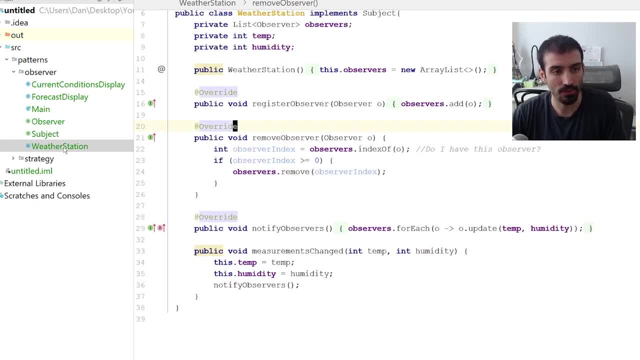 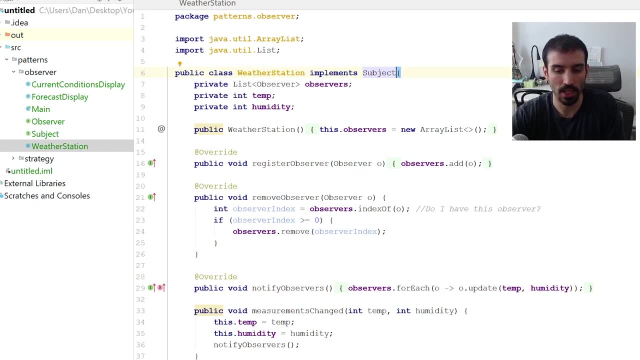 So now, in the context of the subject, let's take a look at the weather station class. So what do we got going on in this class? Okay, so we have a weather station and we see immediately that it implements subject. So that means it must override a few methods. 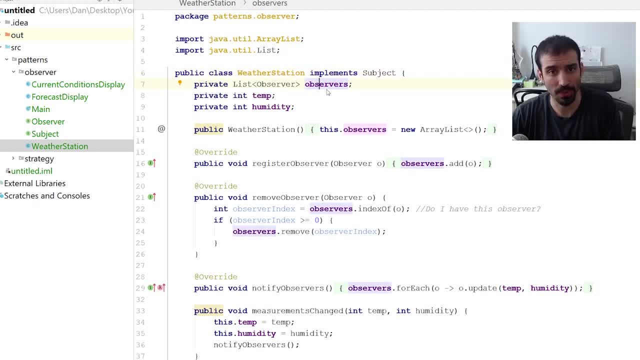 which we'll get to in a moment. We have a list of observers that we're gonna maintain And then, locally, we just keep track of whatever the last recorded temperature and humidity is In the default constructor of this weather station. we're just creating a new array. 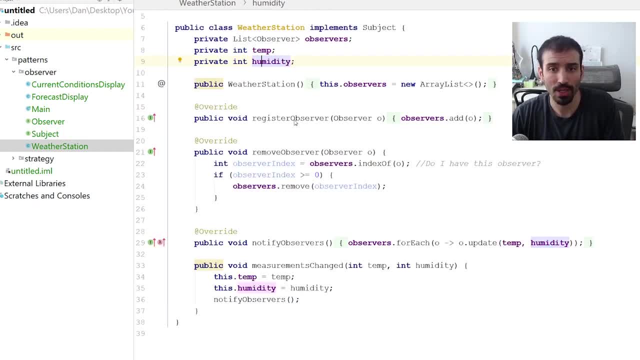 a list for this observer instance And then for the register method, we are just taking in whatever observer that is being passed and adding it to the observer array. Obviously, you may wanna do some kind of deduplication here to make sure you're not adding it twice. 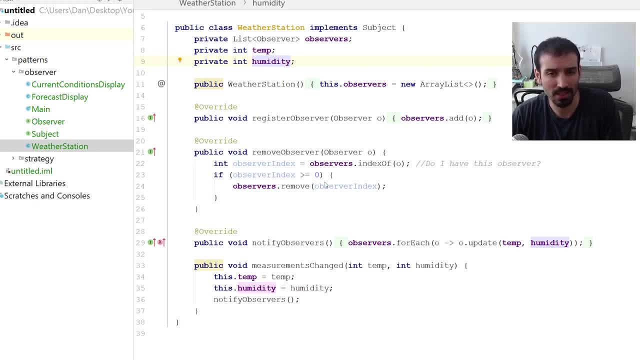 but that's a kind of different thing. For remove it's basically the same thing. The first line here is just figuring out if I have this particular observer in my array already And if I don't, or sorry, if I do rather. 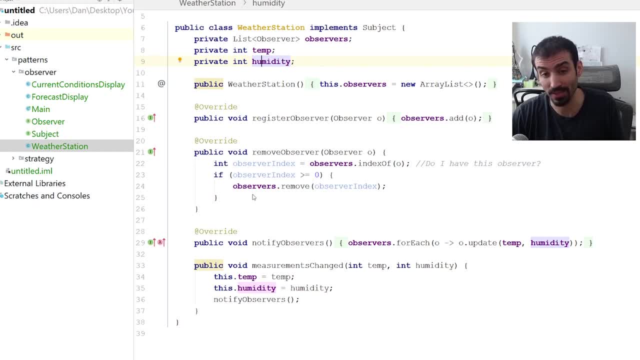 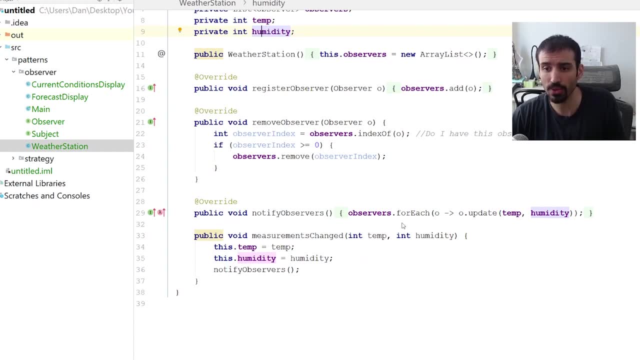 that's what happens. when it's greater than zero, then I need to remove, And if it's not greater than zero, then I do nothing. This method here notifyObservers. all it's doing is it's taking all of my observers and for every one, it's calling the update method. 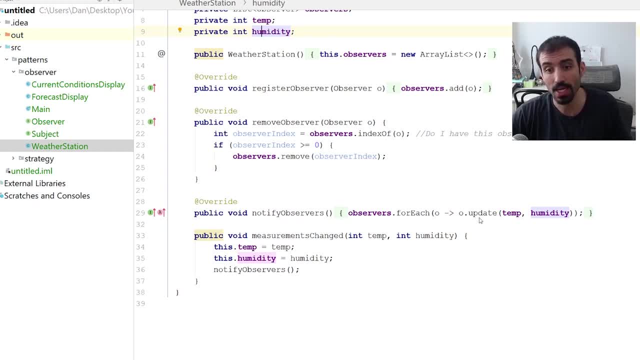 with the temperature and the humidity, Okay, and we're gonna see the implementations of that in the observer classes in a moment, And then, finally, we have this method called measurementsChanged, And this is what is going to be called on the weather station. object: 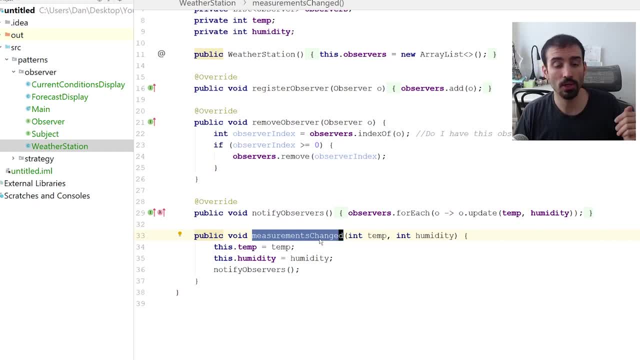 So whenever someone does a recording of that weather station, they're gonna call the weather station's measurementsChanged function, Pass it the new temperature and the new humidity. We're gonna set that locally and then call the notifyObservers method, which is then in turn gonna call. 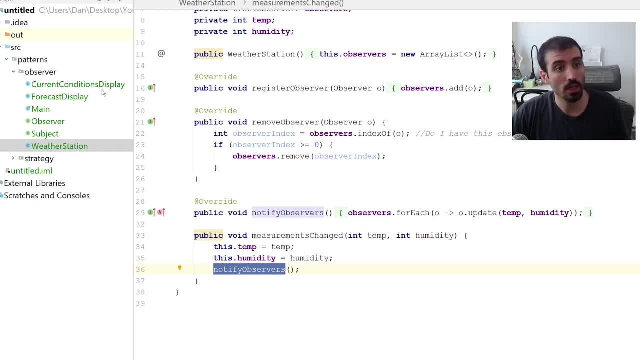 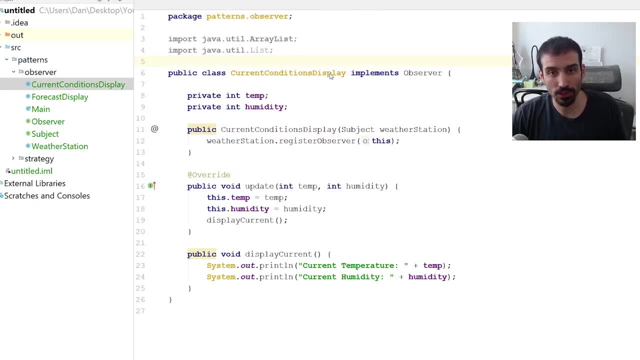 all the observer's update methods. So that's how it's gonna work. So let's go over now to the observers and take a look at the current conditions display. So first of all, note that in this current conditions display class we are implementing the observer class. 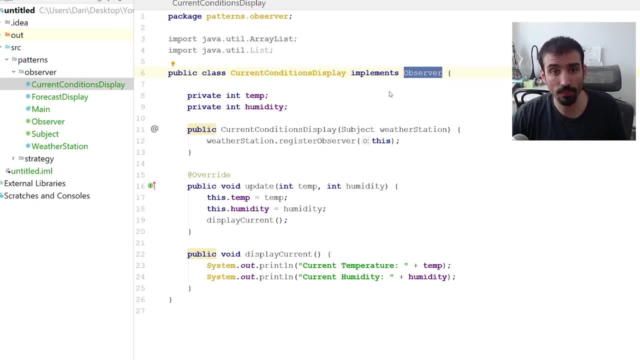 which means that we need to implement the update method as we saw before. We have a local temperature and humidity just to keep track of whatever it is currently In our default constructor. we're taking an instance of the subject, which is the weather station in this case. 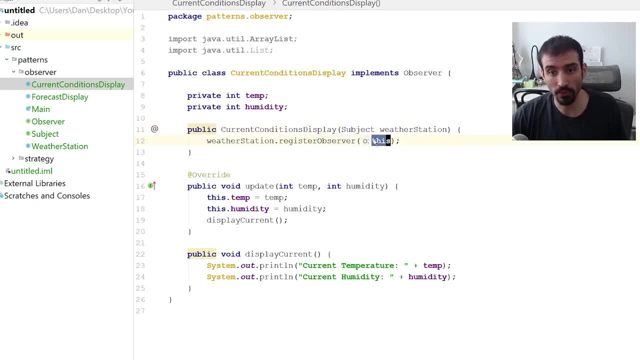 and that's the subject and registering ourselves. So this refers to this instance of the current conditions display class. So we're registering ourselves with the subject And then we just have a update method that takes in the temperature and humidity, sets it to local and then calls the display current. 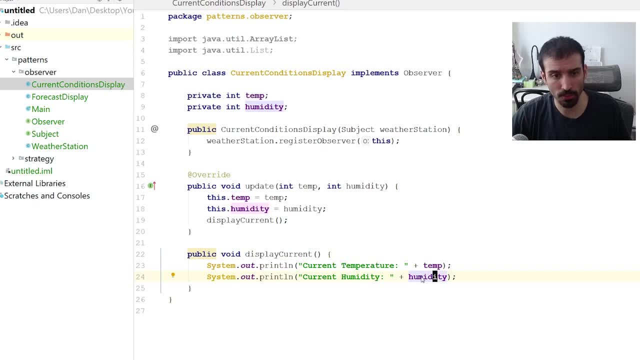 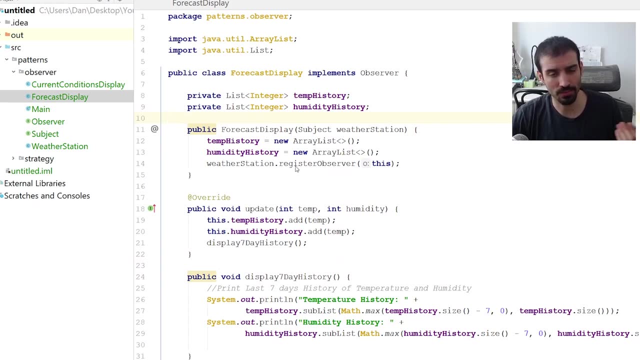 The display current just basically reads the temperature and humidity variables and prints it out to a system out print line. The forecast display is pretty similar, slightly more complicated but almost exactly the same. So forecast display implements observer. we got an array of temperature history and humidity history. 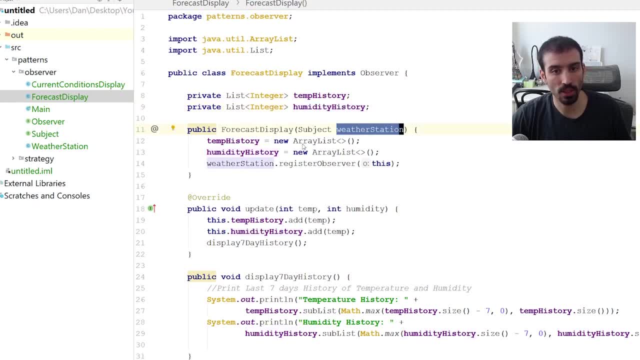 When the constructor is called, we take in the weather station, we initialize the arrays, we register ourselves to be observers for this subject. So we subscribe to the subject or subscribe to the topic And in the update method we add the temperature to our temp history or temperature history array. 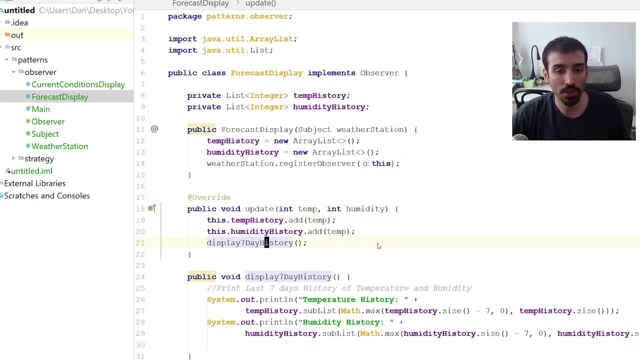 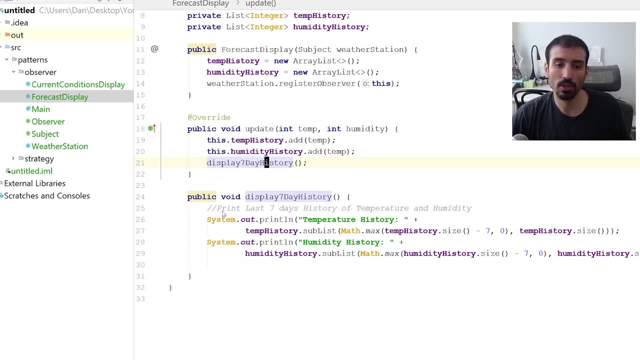 history array. we do the same thing for humidity history and then we call the display seven day history, which all it does is. you know these lines look complicated, but i put a comment here just to make it clear. so these things just print the last seven days of history, for both temperature and 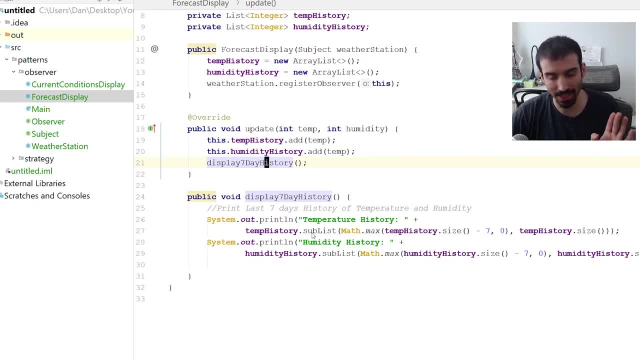 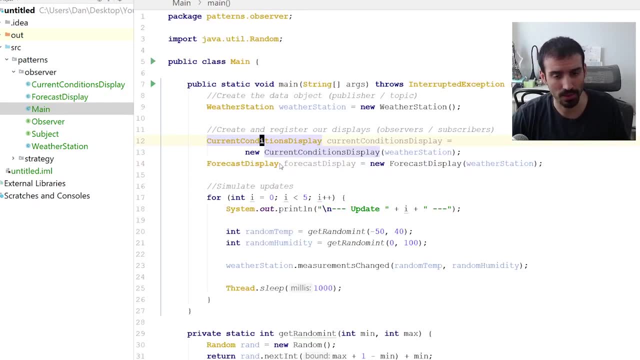 humidity. so it looks complicated, using sublists and math max and all that stuff, but it's really not complicated. so that's all there is to implement the observer pattern. but so let's actually take a look at how this works, like through a runner here. um so the the thing that i wanted to emulate was 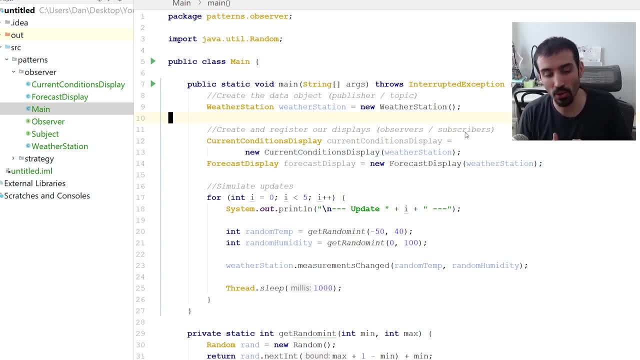 i'm just going to set a timer. every few seconds or every second or so. i'm going to simulate that the temperature gets changed, so like a new measurement is taken and we need to update all of our observers, all of our subscribers. so, taking a look at how i set this up here, so we're creating 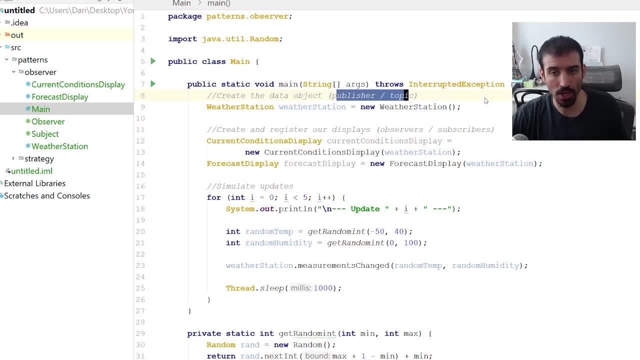 an instance of the weather station which is the publisher or the topic in the pub sub or observer pattern terminology. so we create an empty instance. we need to create and register our displays, which are, in this case, observers. so we're creating a current condition display passing the weather station, creating a forecast- oops, creating a. 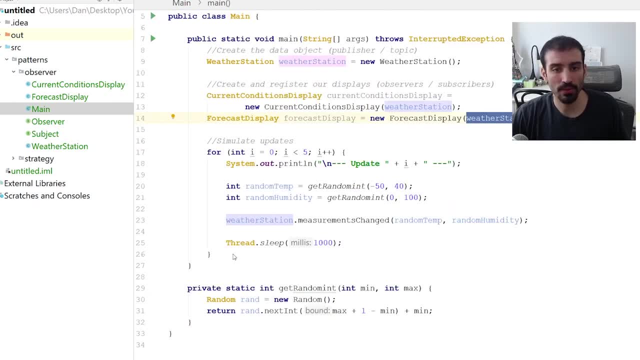 forecast display passing in the weather station, and this is where i'm kind of simulating the updates. so i'm going to do this five times. we're just having a kind of counter thing here that's going to be printed so we can keep track of where we are in the updates, and then we're going to get. 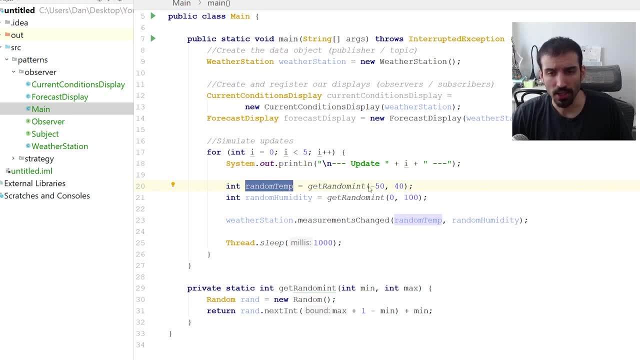 a random temperature here, just making use of this helper function, and it's going to be between the range of minus 50 and plus 40. for humidity it's only between zero and 100, so we're going to be keeping a 100 percent and then, whenever we enter this loop, we're going to say the measurement. 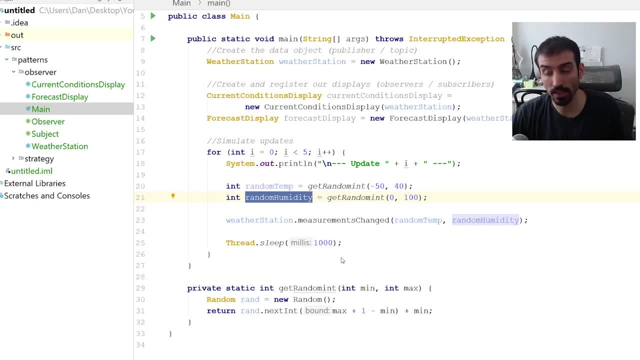 change with whatever these two random values are, and then we're going to sleep and do it again. so that's all. this is so hopefully. if everything works correctly, whenever the measurements change, we should print out the update methods for each of the observers. so let's test that out now to make. 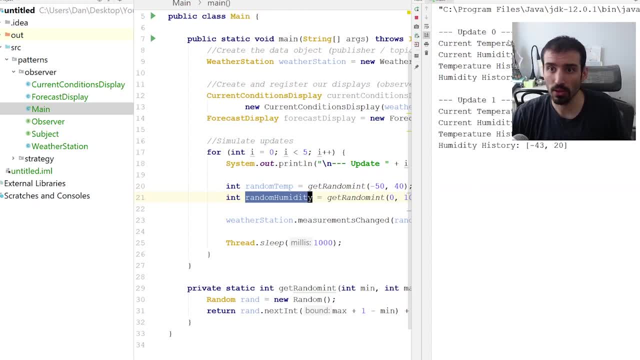 sure this works correctly. so just running it there and we got this going on, so this is looking good. so i only did it. five times zero, of course. so let's just take a look at the output just to confirm. so current temperature was minus 43 degrees. wouldn't want to live there. humidity is 48 and on the first run we have no. 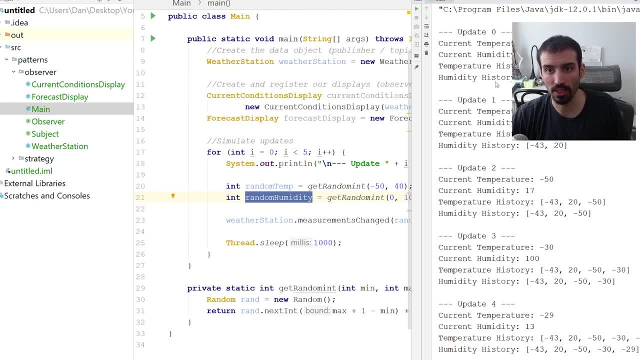 history. so we're just adding it to the temperature history and the humidity history array in that update function and you see, on the next one we actually have the history. so minus 43 took place in update 0 and now the new one is 20.. so you see, with every update here it's growing by one. 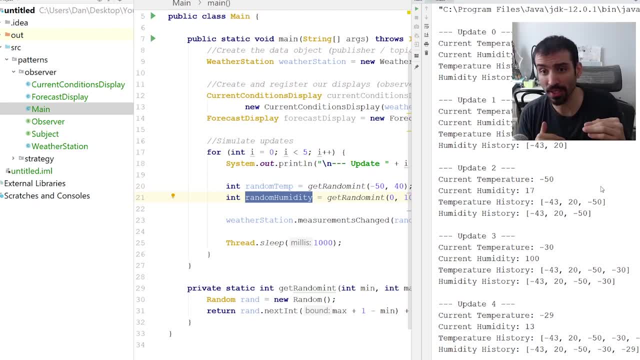 so we can see that everything is working correctly here on every update that's occurring when we call that measurement change function, it's triggering the update function for all the observers. one thing that i do want to note here is like: this is a custom implementation of the. 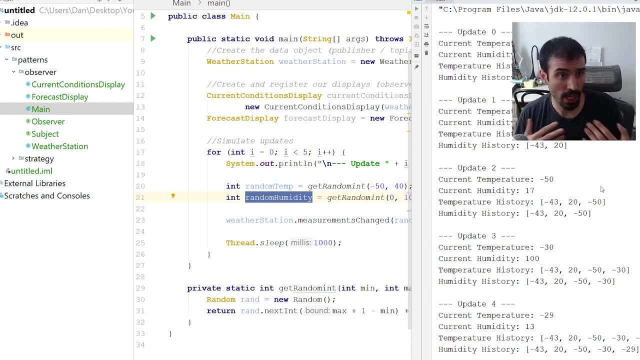 observer pattern. there is by default in the javalang package a observer that you can use, so you don't have to roll your own, you don't have to create these interfaces, and it's got a whole bunch of other more rich features that you can experiment with. but i encourage you to do this exercise. 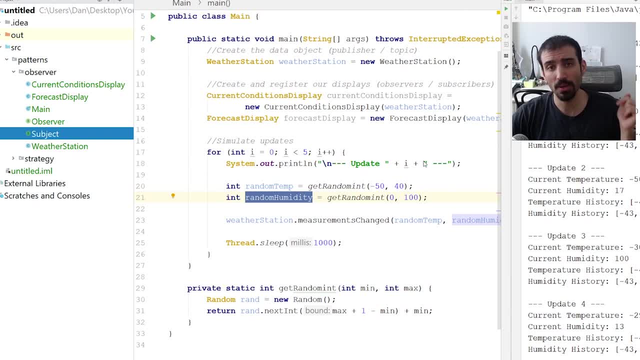 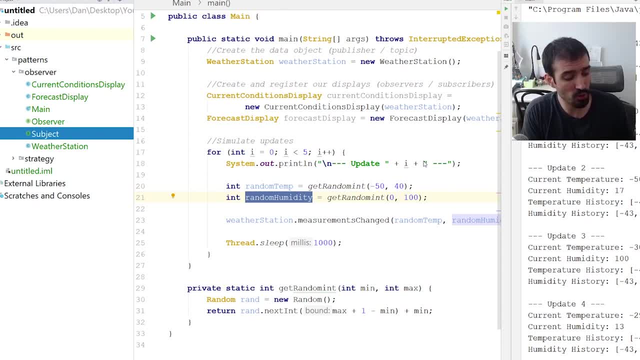 around with it just to kind of strengthen your understanding and if you want to pick up this book, which i highly highly suggest, headfirst design patterns again, i'll put a link in the description section below. so i hope you enjoyed this video, found it useful, learned about the.